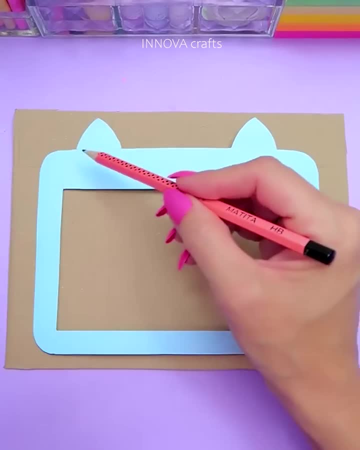 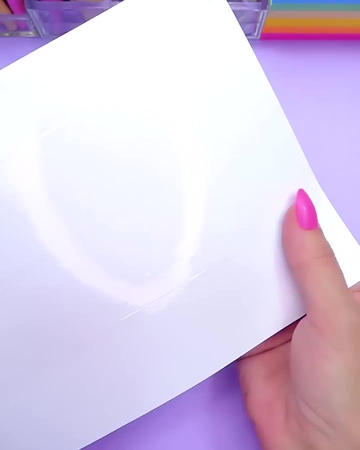 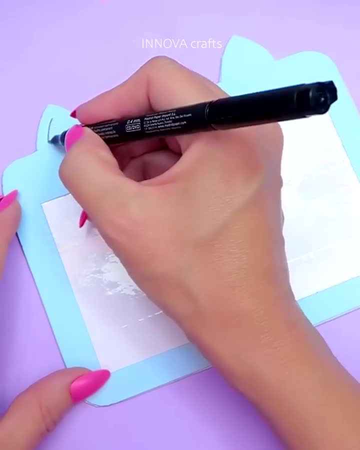 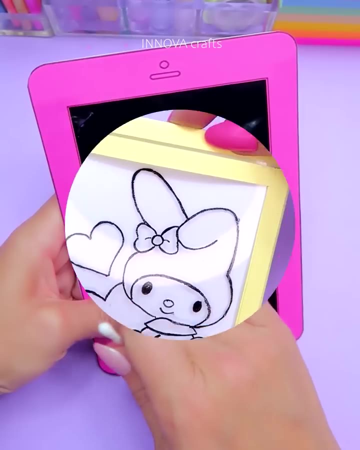 I just wanna hold you. I just wanna look into your eyes and tell you that I want you. You know, you make me feel so alive. Can't stop thinking about you day and night. Love it when you kiss me, love it when you touch. 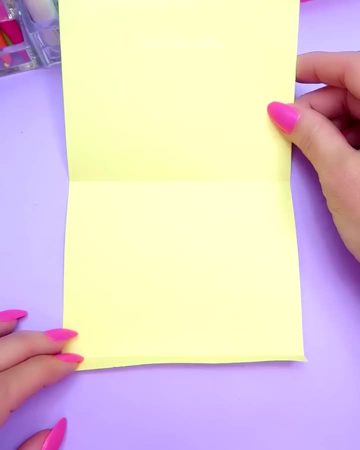 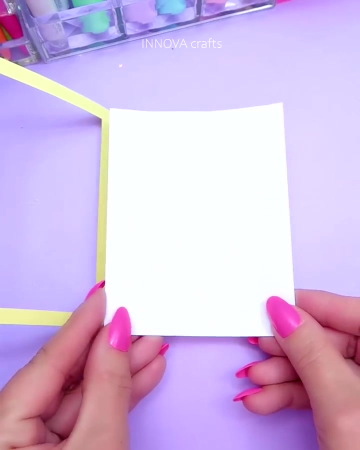 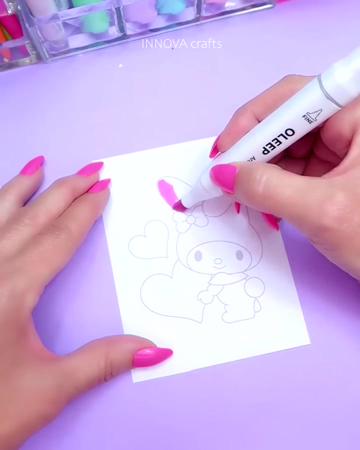 Love the broken, Love the broken, Love the broken. I'm the one calling all the shots, shots, shots. Whether you're ready or not, I'm about to pump this place up, up, up. I'm the cool kid from the back. I'm the one calling all the shots, shots, shots. 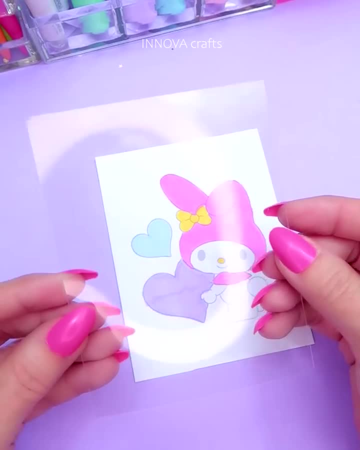 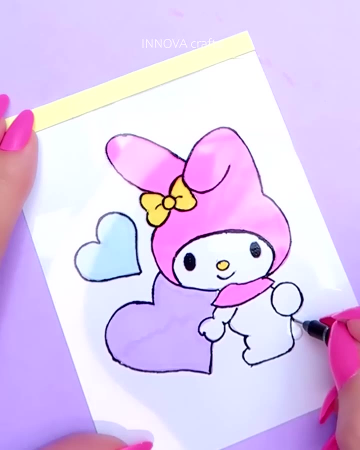 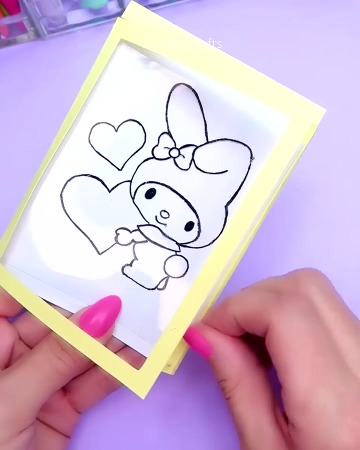 Whether you're ready or not. I'm about to penalty drop. I'm the cool kid from the back. I'm the one calling all the shots, shots, shots. Whether you're ready or not, I'm about to pump this place up, up, up. I'm the cool kid from the back. 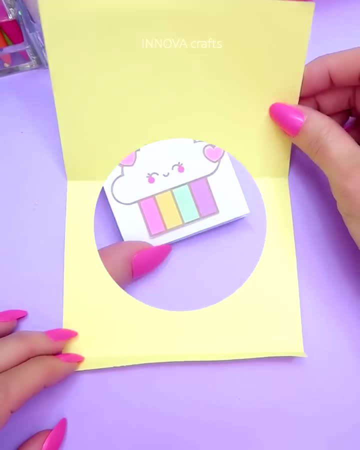 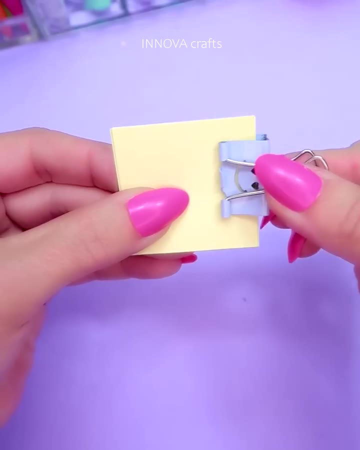 I'm the one calling all the shots, shots, shots. God, I'm in faith, God, I'm in faith. I wanna make you feel good. Trap on me, babe. trap on me, babe. Play a record, feel smooth. Don't know what time, but it was late. 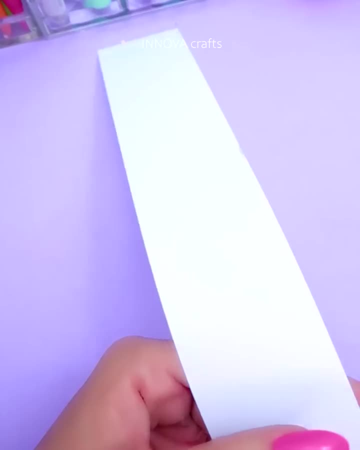 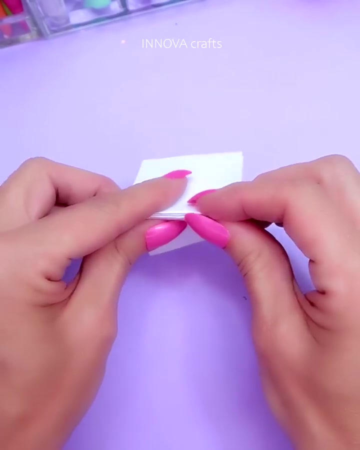 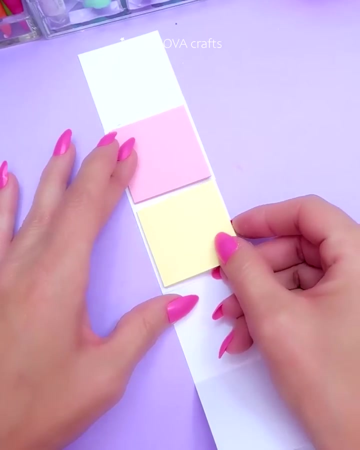 When I met you and your little mate Had some wine love for you a sip. I was so high, but I remember it. I know I was right That these are just feelings, But these ones, they feel like they For just one reason: God, I'm in faith. God, I'm in faith. 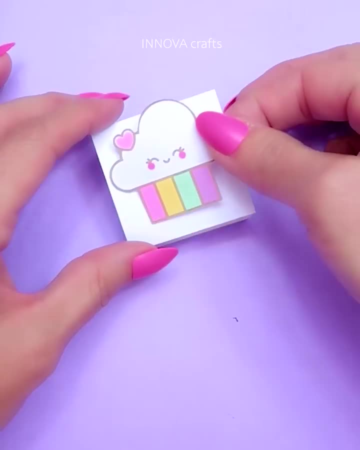 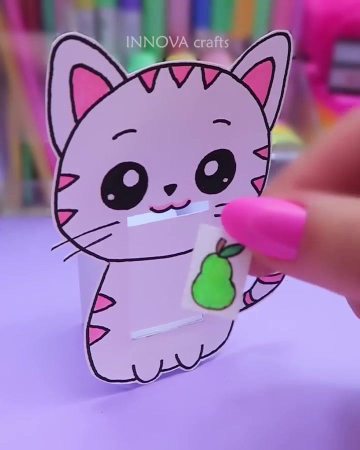 I wanna make you feel good. Trap on me, babe. trap on me, babe. Play a record, feel smooth. Don't know what time, but it was late. God, I'm in faith. God, I'm in faith, I wanna make you feel good. 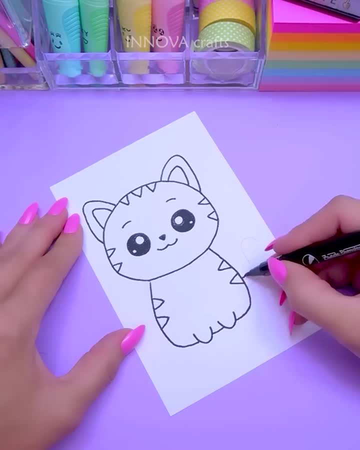 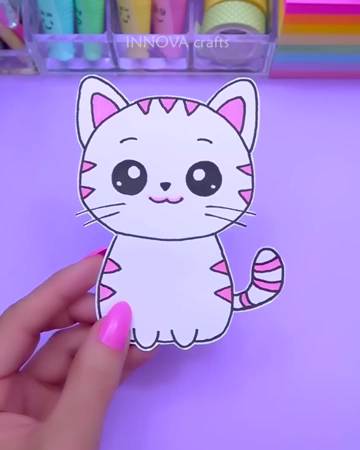 Trap on me, babe. trap on me, babe. Play a record, feel smooth. Don't know what time, but it was late When I met you and your little mate Had some wine. love for you a sip. I was so high, but I remember it. 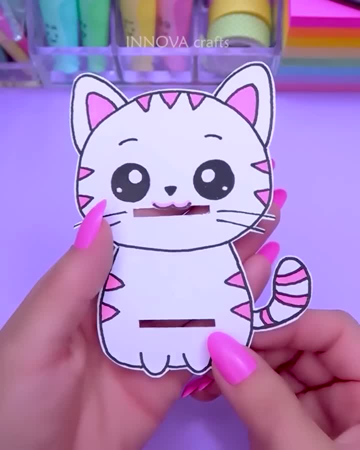 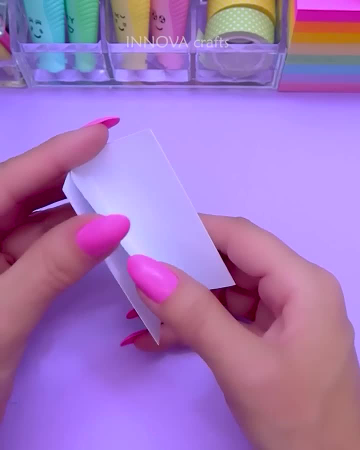 I know I was right That these are just feelings, But these ones they feel like they For just one reason: I wanna make you feel good. Trap on me, babe. trap on me, babe, Play a record, feel smooth. Don't know what time, but it was late. 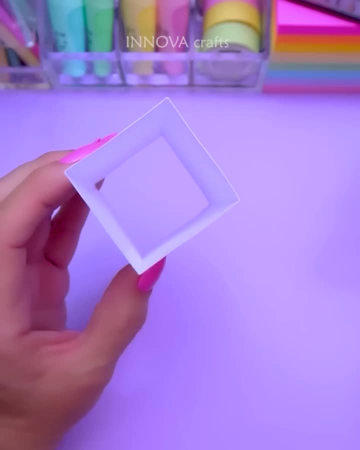 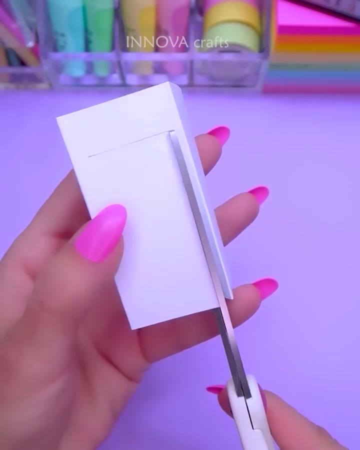 They feel like they for just one reason: Fly on me, babe. fly on me babe. I wanna make you feel good. Trap on me, babe. trap on me babe. Play it, break it feel smooth. Fly on me, babe, fly on me babe. 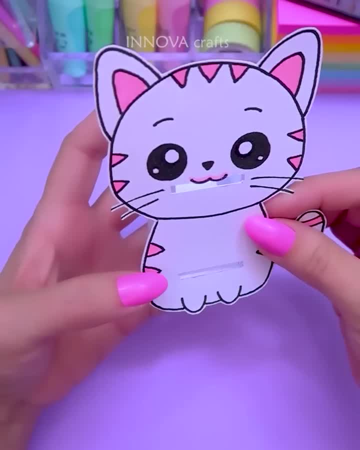 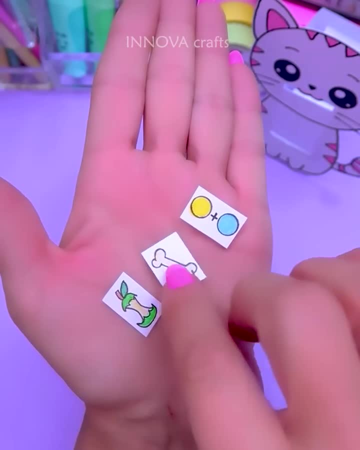 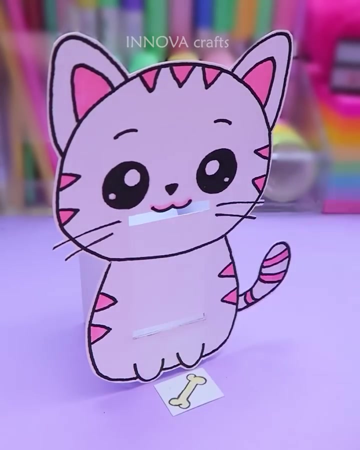 I wanna make you feel real good. Trap on me, babe. trap on me, babe. Play it, break it feel smooth. So we took a ride, One last bite, with the best kind of sight. Plenty of us walked away at a time And the city made me realize. 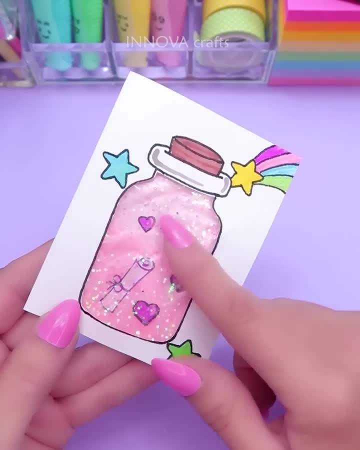 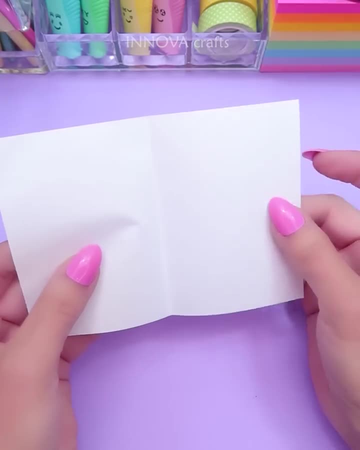 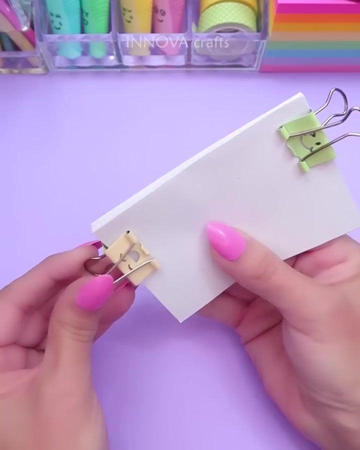 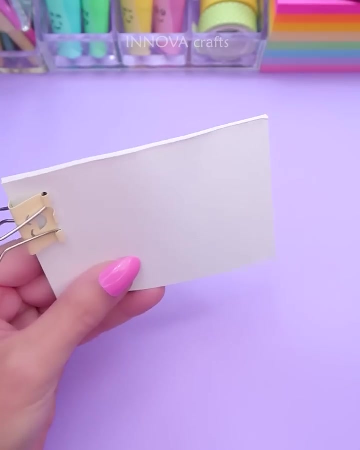 I know I won't let go. This is what it's like. I could get used to late nights Dancing my place. I could get used to long drives Can't rise your place. I could get used to be fighting Just for the hell of it And you're putting up with it. 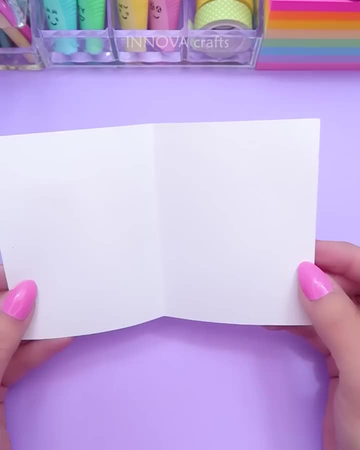 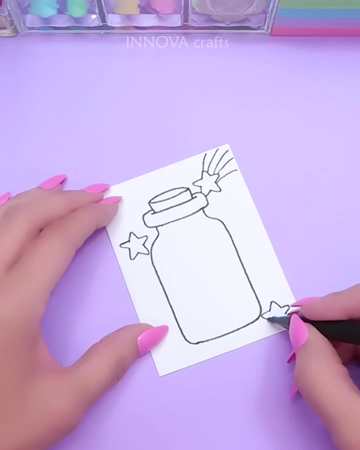 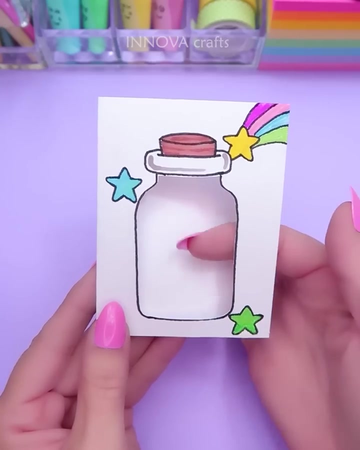 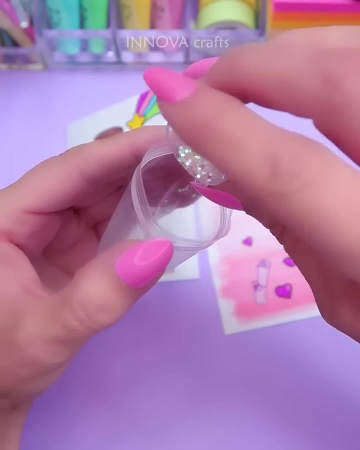 Cause you're the meat of this. Late nights dancing our place. I could get used to this. I thought it would scare me. I thought it would scare me to let you in, But I was paper thin. You saw right through me And I gave in. My mind was occupied. And then I was on a high Could run forever to get a minute, Just a minute of your time. If this is what it's like, I could get used to late nights Dancing my place, I could get used to long drives Can't rise- your place I could get used to. 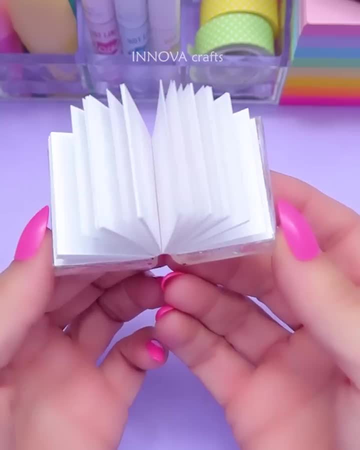 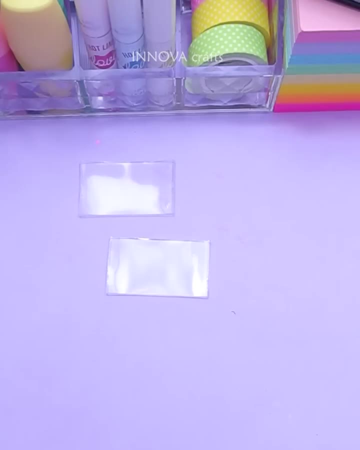 I could be raw, I could be tall. I'll make you feel real uncomfortable. I can give you my thing, But not my hand. I won't do your silly little dance. Don't need hugs. Done with the chalk. I know your next move. I can pick on Moving fast. 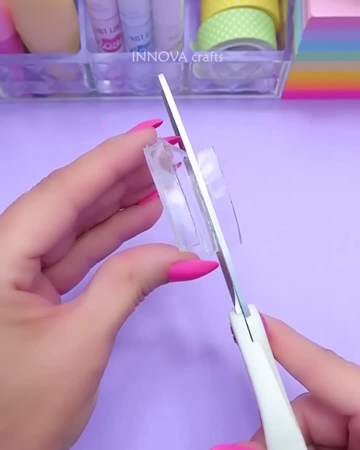 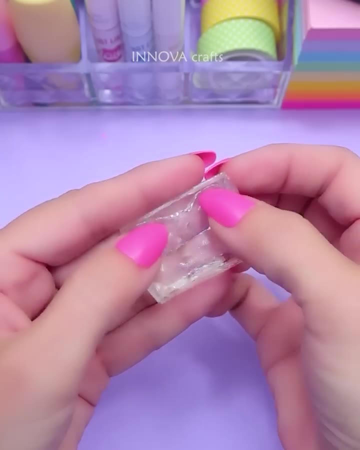 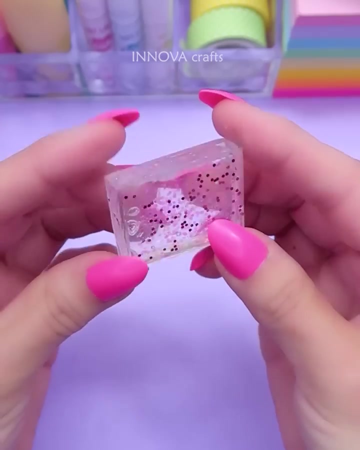 Catch, if you can, When I'm happy you can't stand it. Maybe high, then low. Told me, let's take it slow. Next thing that I know You got a next best hope: Summer soon. body snows, yeah, Soon too. you'll find out that. 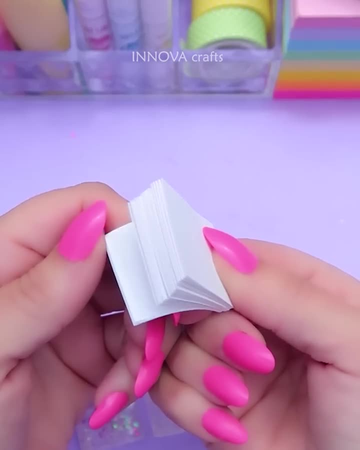 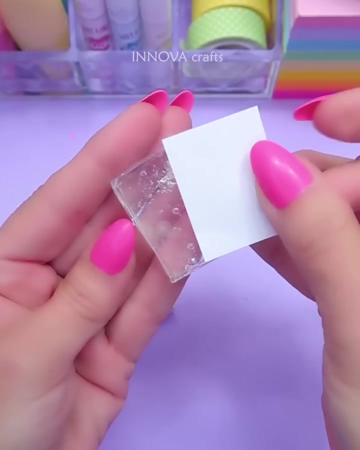 But you just wanna roll And all I think is whoa. Weekends spent in the studio, Weekdays crowded like bros. I think back and it's obvious, Obvious, so obvious. I could be raw, I could be tall. I'll make you feel real uncomfortable. 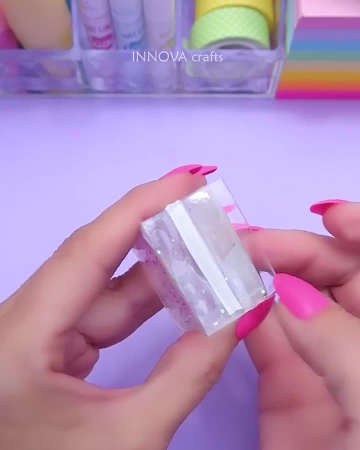 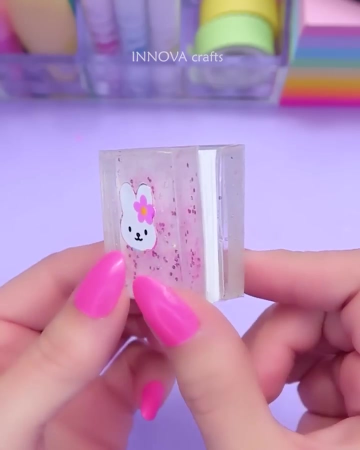 I can give you my thing, But not my hand. I won't do your silly little dance. Don't need hugs Done with the chalk. I know your next move. I can pick on Moving fast, Catch, if you can, When I'm happy. you can't stand it, So you call my money. 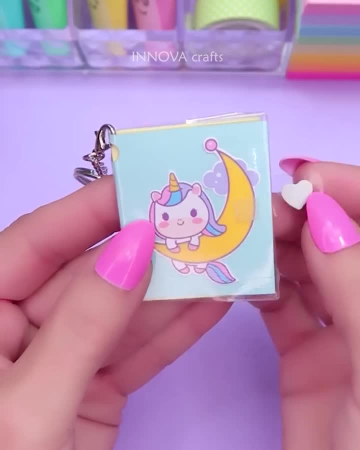 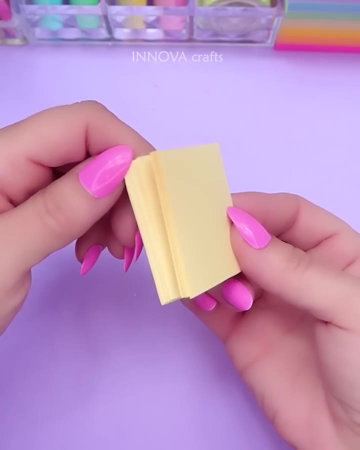 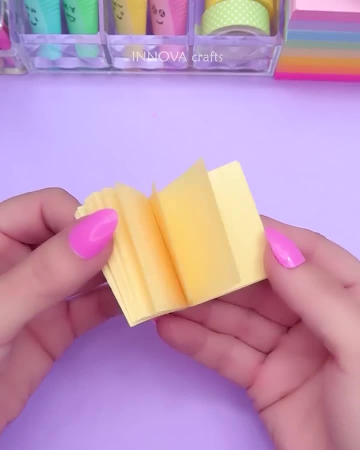 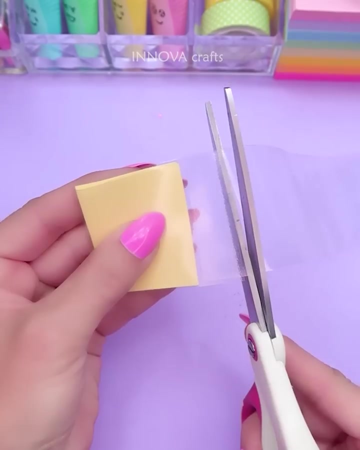 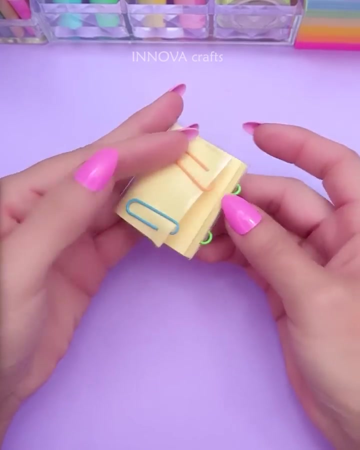 Don't know what time, but it was late. When I met you and your little mates Had some wine. offer you a sip. I was so high, bright, remember it. I know I was right That these are just feelings, But these ones they feel like they. 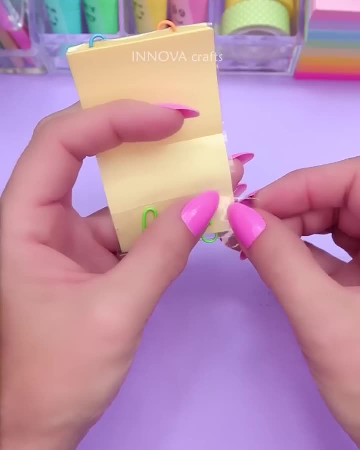 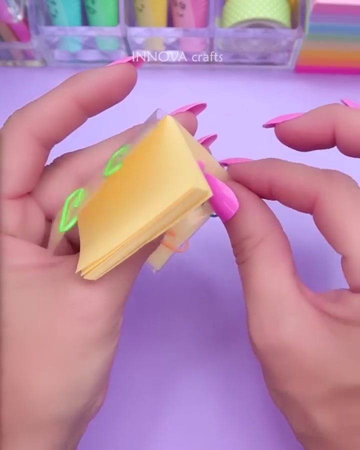 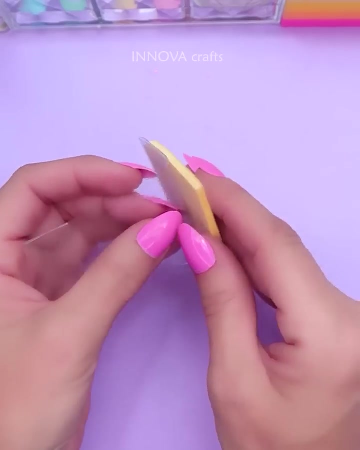 For just one reason: Sly on me, babe. sly on me, babe. I wanna make you feel good. Trap on me, babe. trap on me babe. Play a record, feel smooth. Sly on me, babe. sly on me babe. Sly on me, babe, trap on me babe. 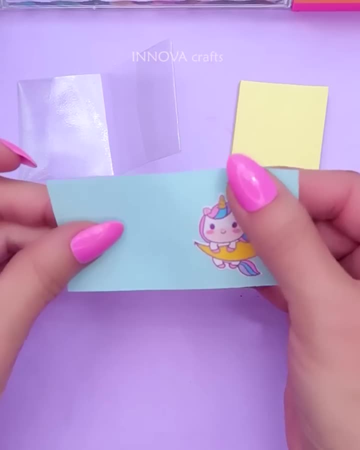 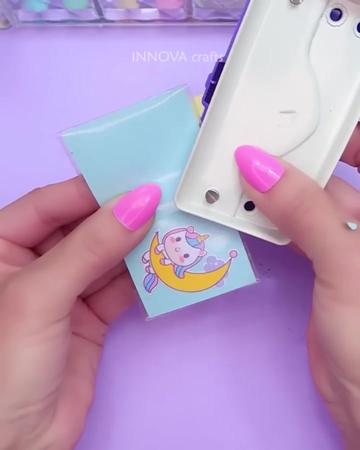 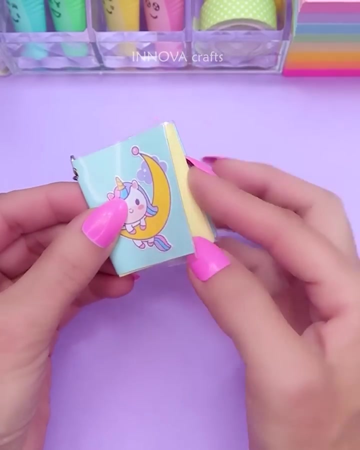 I wanna make you feel good. Trap on me, babe. trap on me, babe. Play a record, feel smooth. So we took a ride One last bite with the best kinda side. Funny how we smoked away all the time And the city made me realize I know I was right. 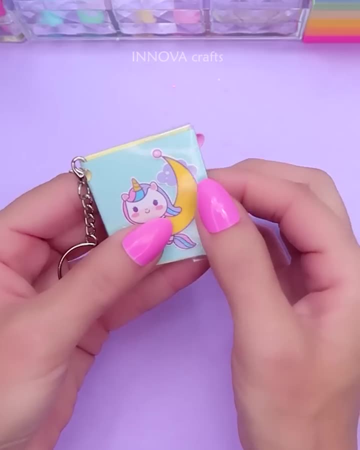 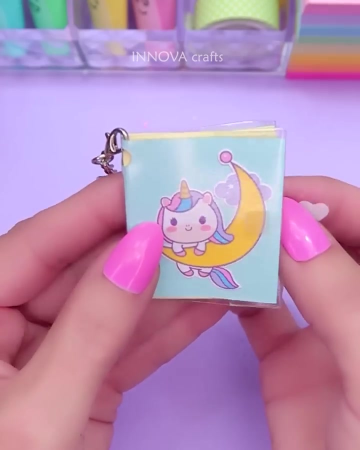 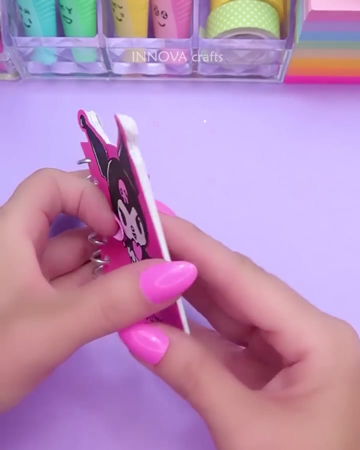 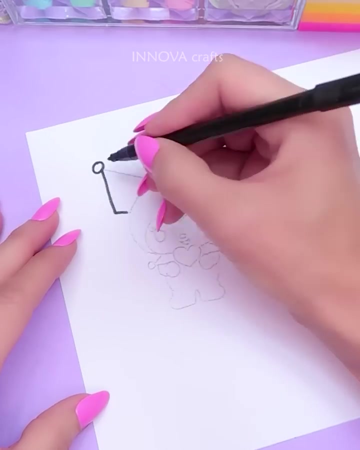 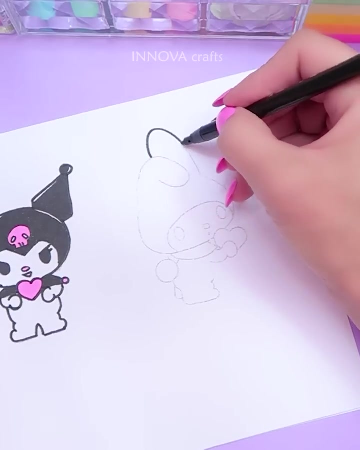 That these are just feelings. But these ones, they feel like they, For just one reason. I won't make it easy for you now. You got two minutes of my time And I don't really break too easily, But I'm worth it, cause I'll slip into your dreams tonight, oh So give me, so give me your all. 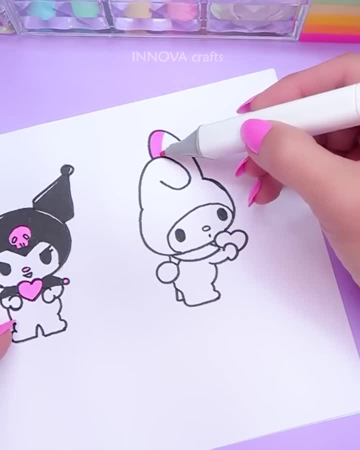 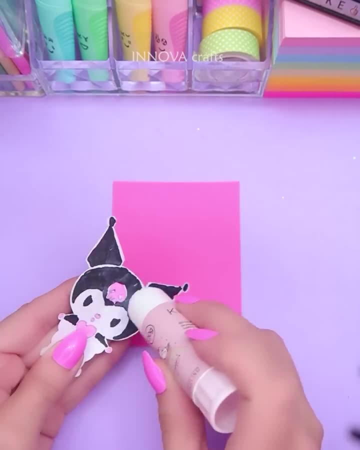 I'll take it. I'll take it to Mars. oh, I'll stick like glue inside your mind. Just watch me break in. you'll see You're falling into me. touch me. I swear You would do anything that I want. So keep us awake till the dawn. oh, 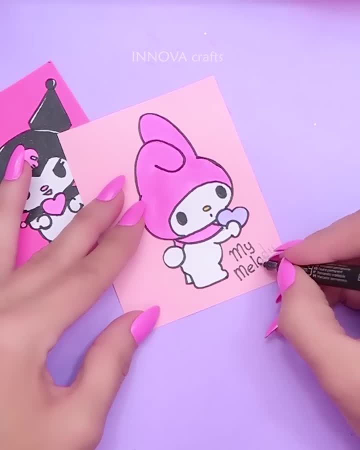 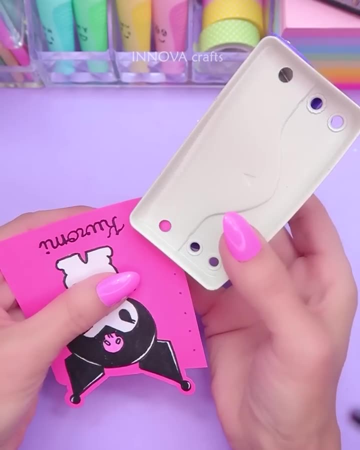 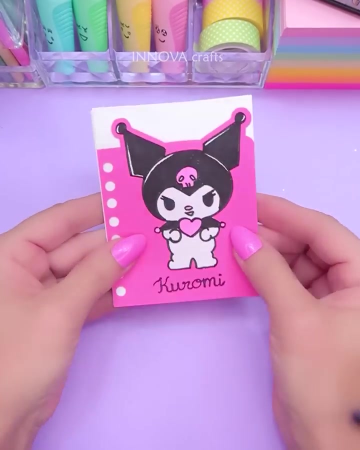 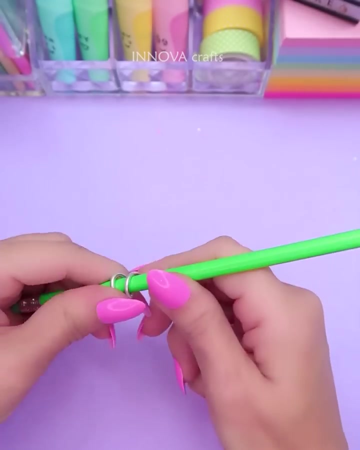 Baby, we're free. I wanna make you sweat on me. I wanna make you sweat on me. I got you wrapped around my finger, But don't you try to call me tomorrow. There's nothing personal in heaven. I'll let you go. You got two minutes of my time And I don't really break too easy for you now. 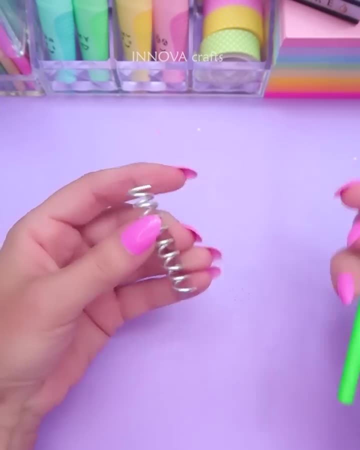 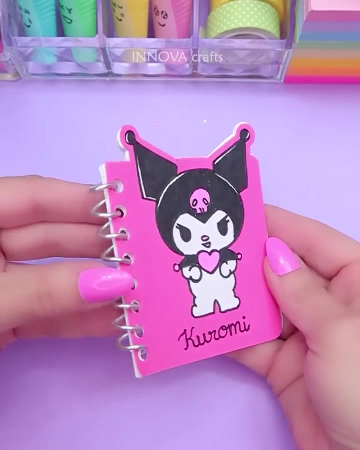 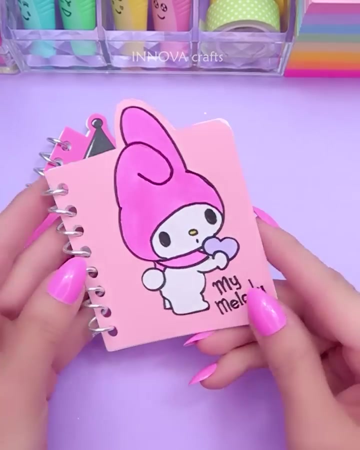 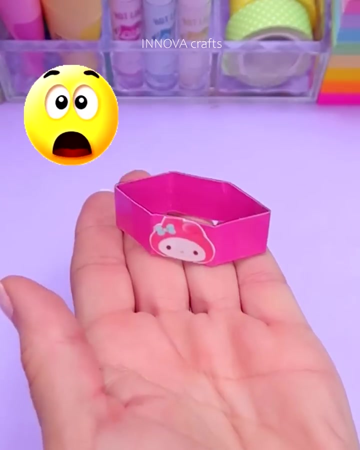 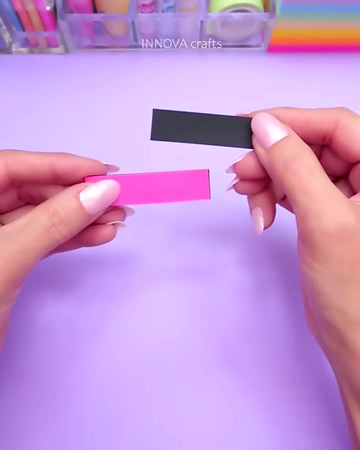 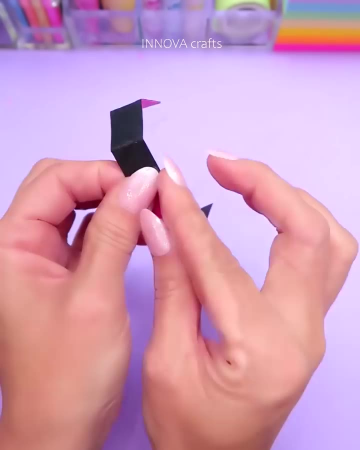 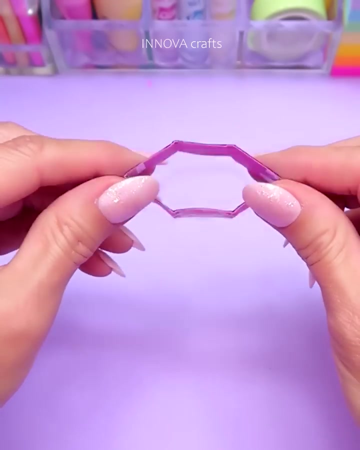 Whether you're ready or not. I'm about to pump this place up, up, up. I'm the cookie from the bucket, I'm the one calling all the shots, shots, shots. Whether you're ready or not, I'm about to penalty drop. We're spinning, spinning on a loop all night. 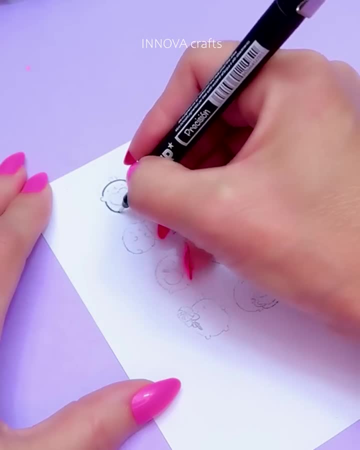 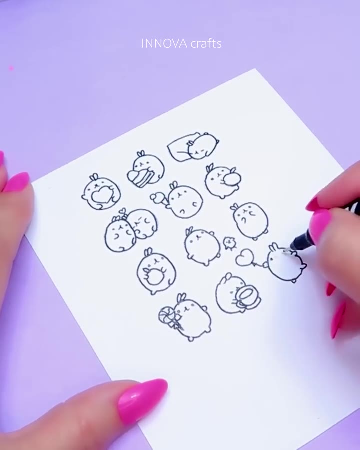 Slide on me, babe. slide on me, babe. I wanna make you feel good. Trap on me, babe. trap on me, babe. Play a record, feel smooth. Don't know what time, but it was late When I met you and your little mate. 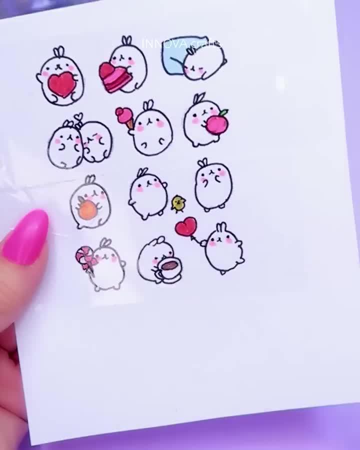 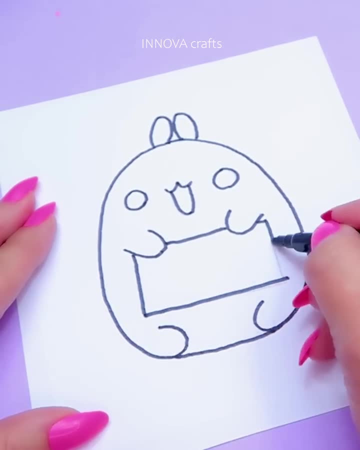 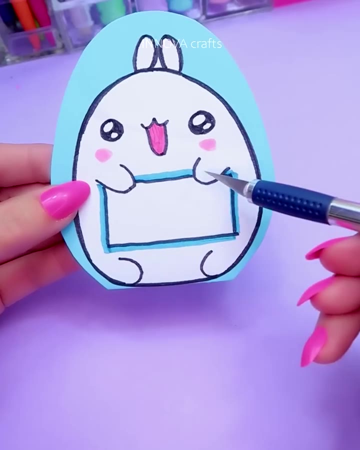 Had some wine. love for you a sip. I was so high, bright, remember it. I know I was right. But these are just feelings. But these ones, they Feel like they Fall just for reason. Slide on me, babe. slide on me babe. 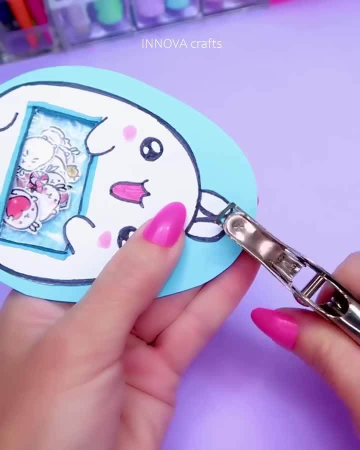 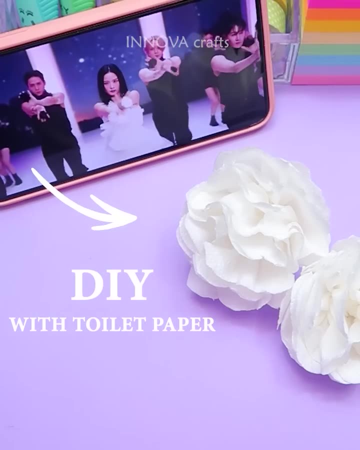 I wanna make you feel good. Trap on me, babe. trap on me, babe. Play a record, feel smooth. Don't know what time, but it was late. I'm the one calling all the shots, shots, shots, Whether you're ready or not.